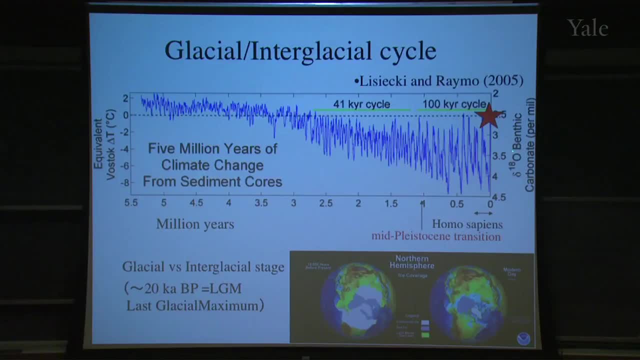 And this is a kind of stack of many deep sea cores. so it's not just noise- and people start to see particular cycles. that's dominant 41 kilo year cycle from one to two million years and the last one million years dominated by 100,000 year cycle. 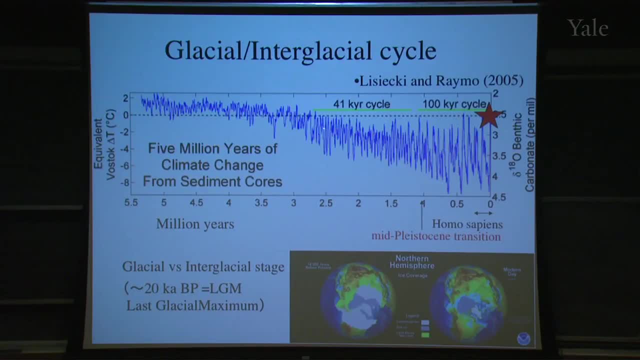 Also the interesting thing is that you know, in the past we've been talking about, you know the interesting features- that the amplitude has changed and also the average level has changed And this is thought to be a kind of proxy of sea level or ice volume. 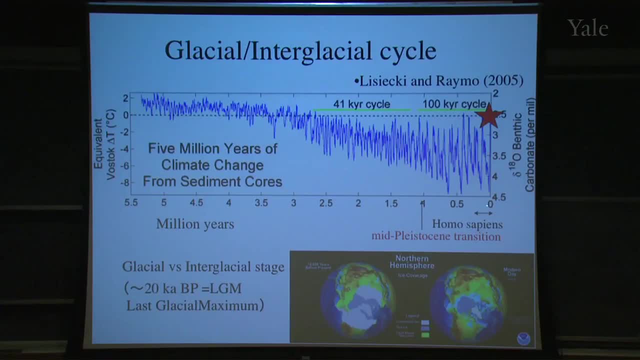 So the larger ice volume means that the isotope shifts downwards, or a larger number, And present day is at this level with the big red star. So you see that the level, the same level of present days, is coming every year. It's coming every about 100,000 year cycle for the one million years and also an average. 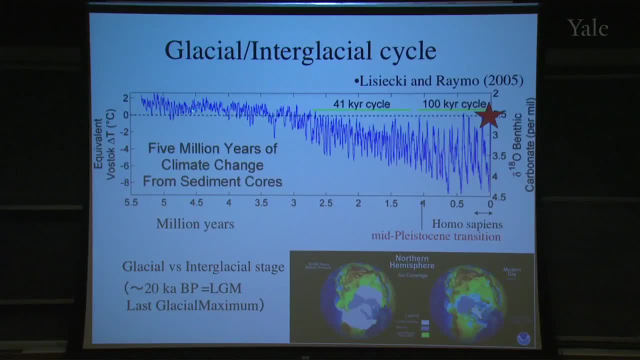 back to three million years, so-called pliocene, which Trude, I think. she skipped this topic, unfortunately, but I hope to discuss with her later. Anyway, Today's topic is try to model and understand The difference between the glacial and interglacial cycle and the mechanism of the 100,000 year. 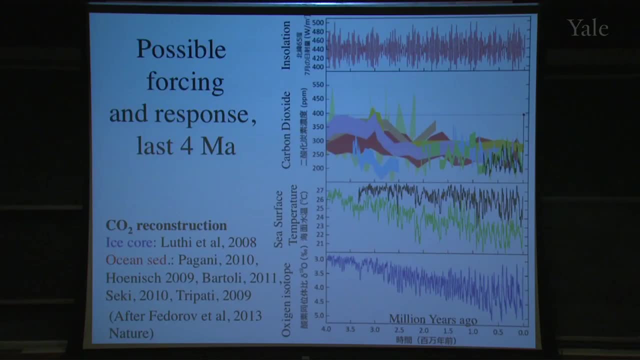 cycle. Possible forcing and possible forcings that are involved, or people think that is involved, is this so-called Milankovitch cycle, or this is in terms of summer insulation of the high latitude, ranging from 400 to 500 watt per square meter. So about changing. 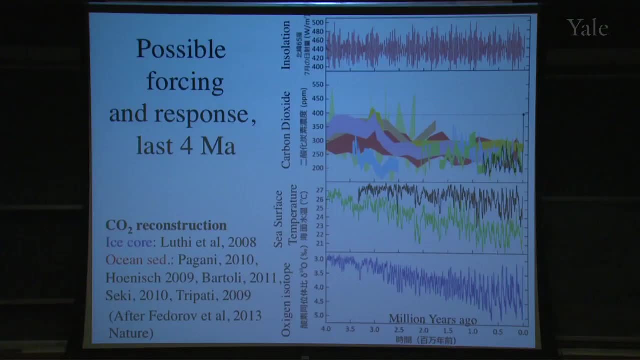 Changing for about 20, 20% of the summer. solar radiation And also the greenhouse gas has changed here and was compiled here by Alexey Fedorov in this department, including the data from Professor Pagani, And we see we start to see some fruitful information in the past of the carbon dioxide. 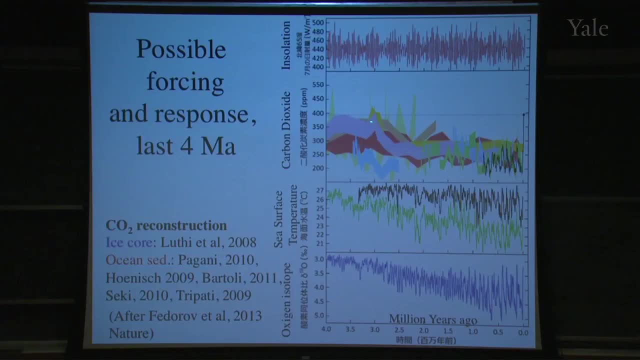 which is which was About Between 300 and 400 PPM before 2 million years ago And now below 3 million- 300 million, and also excellent match with the ice core and ocean sediment information in the past 800,000 years. 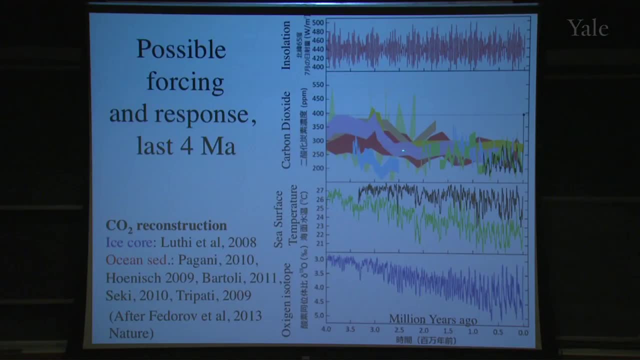 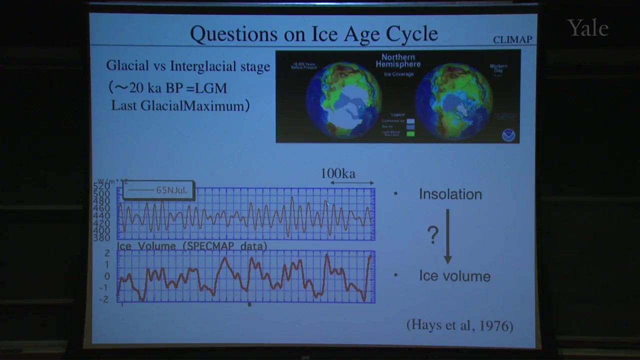 So we have a slight idea that greenhouse gas and insulation could change And Have Influenced the climate and the ice volume and resulted in this curve, But how it this was how this happened is not still not clear For the past 400,000 years, especially if we think the insulation is the driving force. 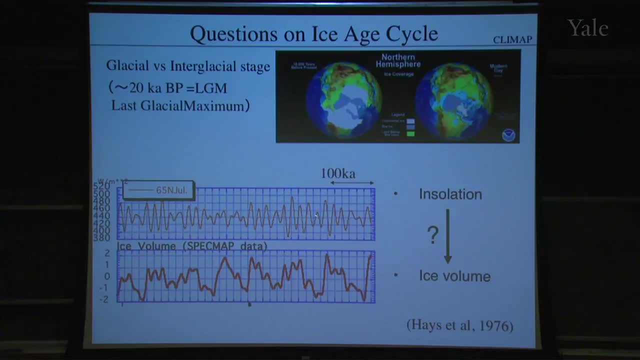 One puzzle is that the 100,000 year cycle is not seen in the insulation, seen in the insolation spectra, It's mainly the 21 and 23, about 20,000 year cycle, which is the cycle of the position of the Earth. 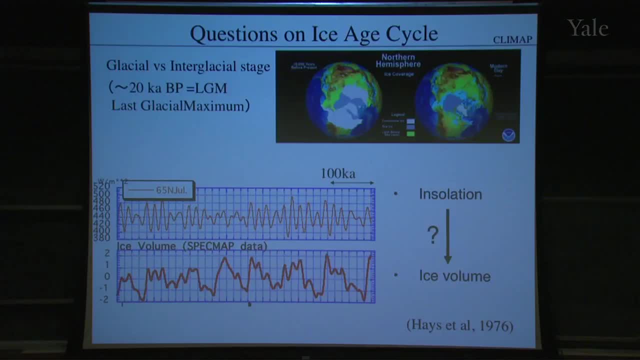 seasonal march of the Earth. on Earth orbit around the sun. That makes the summer amplitude large, because of some eccentricity And also the obliquity which is because of the tilt of the axis for 40,000 years. you can see. 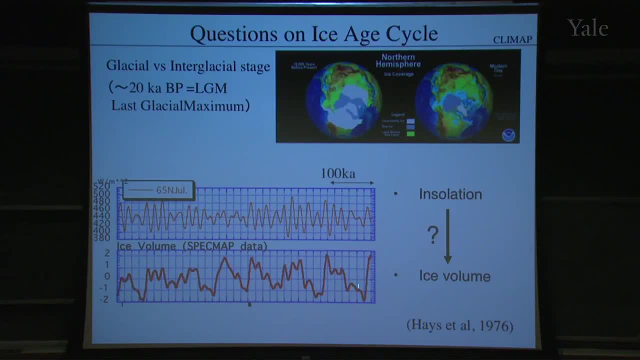 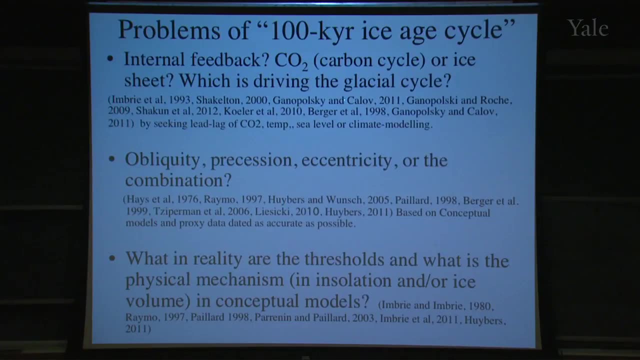 But the dominant cycle for the ice volume or the climate is the 100,000 years cycle. So the problem of this ice age cycle, so-called 100 kilo year ice age cycle, is: what is the mechanism? And we need some kind of internal feedback. 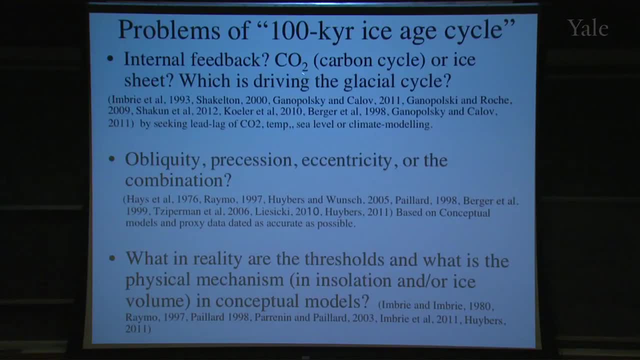 Candidate is the recent data that shows very beautiful match of 100,000 year cycle to the by the carbon dioxide in the atmosphere retrieved from ice core bubbles. But also the ice sheet itself is a candidate to make a long term to.